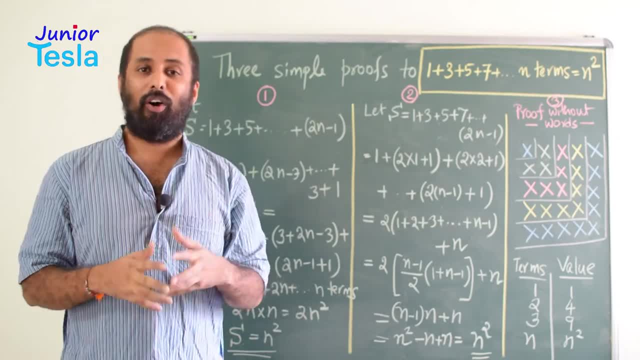 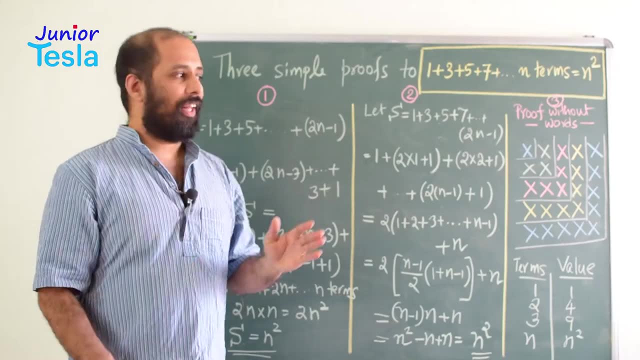 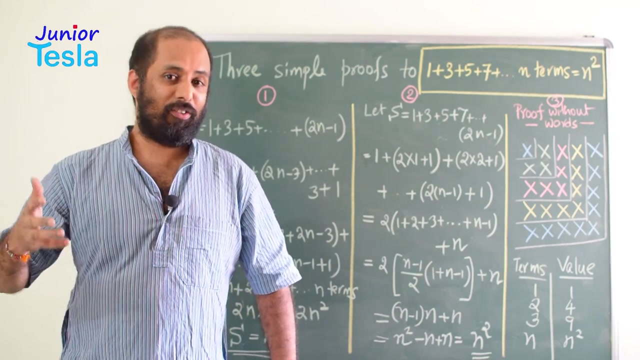 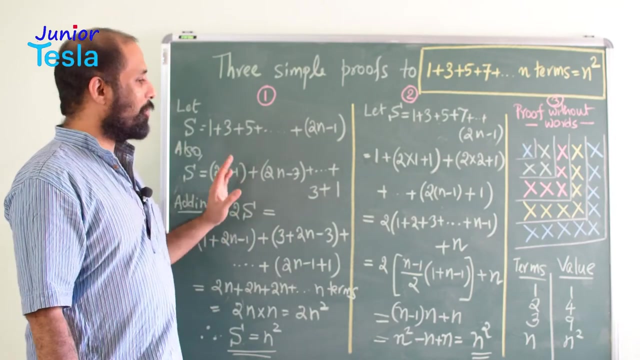 numbers, the sum should be n square. Now how do we prove this? We have taken 3 very simple proofs to prove that the sum of n odd natural numbers is equal to n square. Let us see how to do it In the first method. what I am going to do is: I have taken 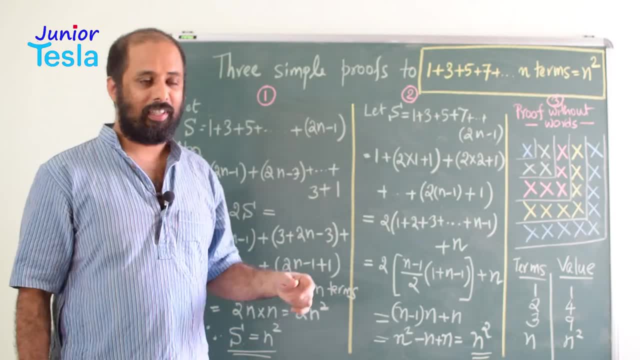 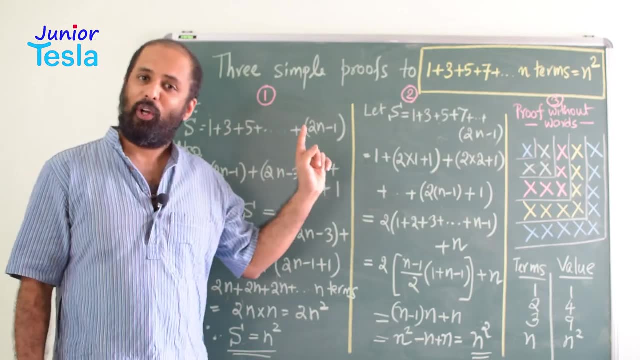 yes, I have denoted the entire series as yes. Now what is that series about? It is sum of n odd natural numbers, That is, 1 plus 3 plus 5, etc. up to 2n minus 1.. So if you have taken n, 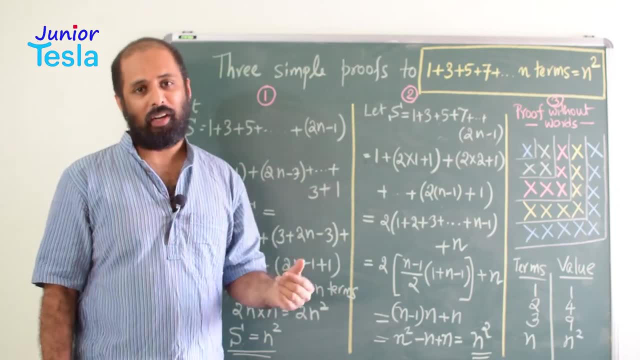 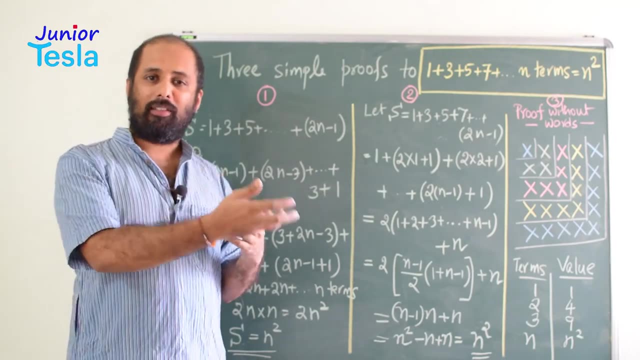 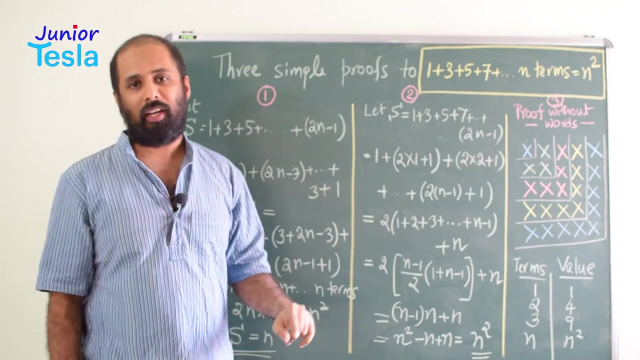 odd natural numbers. the nth term will be 2n minus 1.. Now let me take the same series. yes, but let me write the terms in a different way. I will take the last term first and the first term last. That is 2n minus 1 plus 2n minus 3, plus 2n minus 5, etc. up to 1.. Now I am going to add: 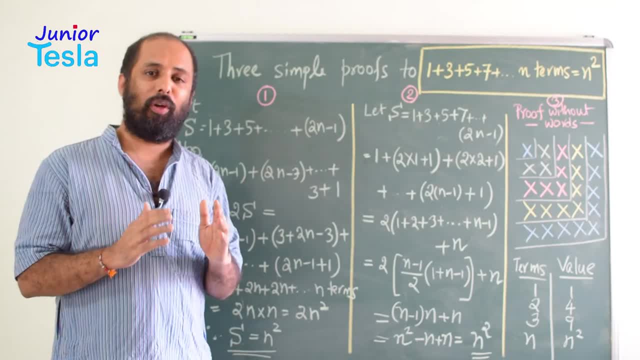 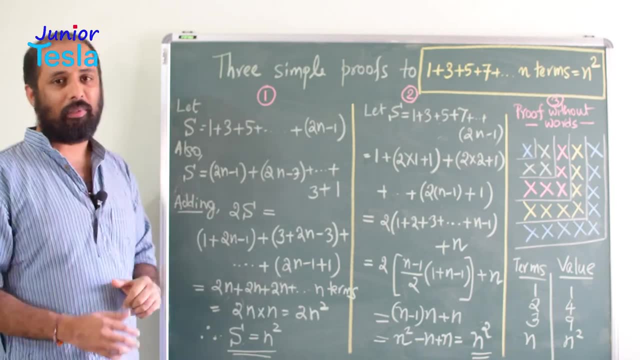 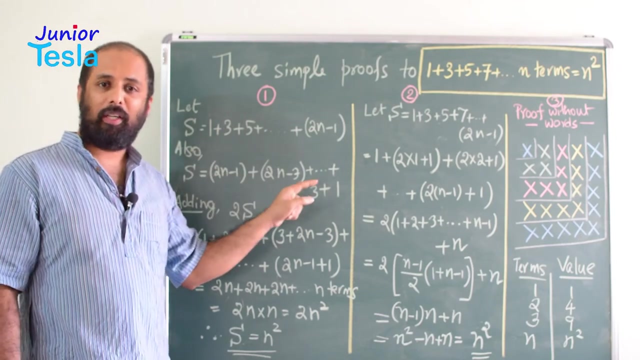 these two lines. Since it is the same equation, I am going to add these two lines. In the left hand side, I get yes plus yes, which is equal to 2, yes. And on the right hand side, what happens? Let us see: 1 plus 2n minus 1, 3 plus 2n minus 3, 5 plus 2n minus 5, 7 plus 2n minus 7, etc. 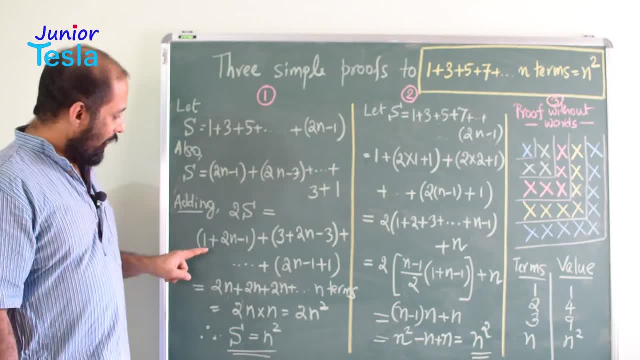 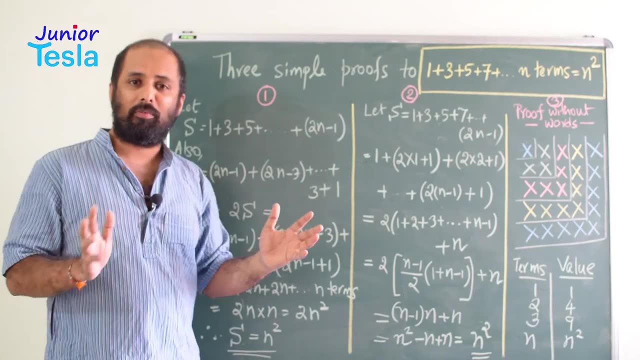 up to 2n minus 1 plus 1.. Now here all these first and third terms. they get cancelled. So 1 minus 1, 3 minus 3, 5 minus 5.. All those terms will get cancelled and what is remaining is 2n. 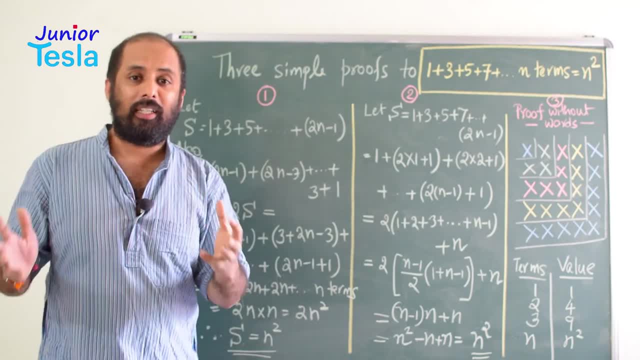 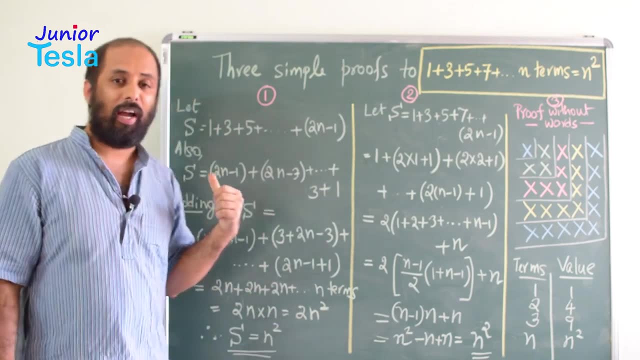 plus 2n, plus 2n, plus 2n, etc. Totally n terms 2n. So it is nothing but 2n into n, which is equal to 2n square. Now remember, in the left hand side you have added yes plus yes, So. 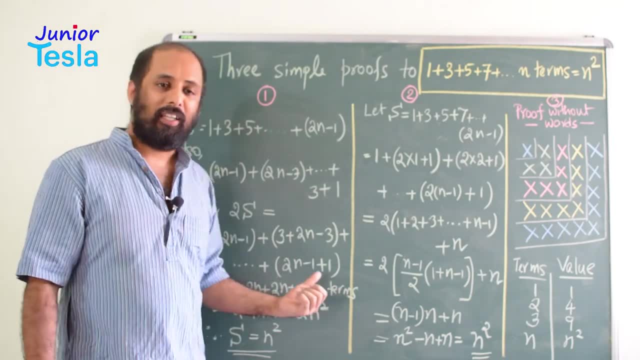 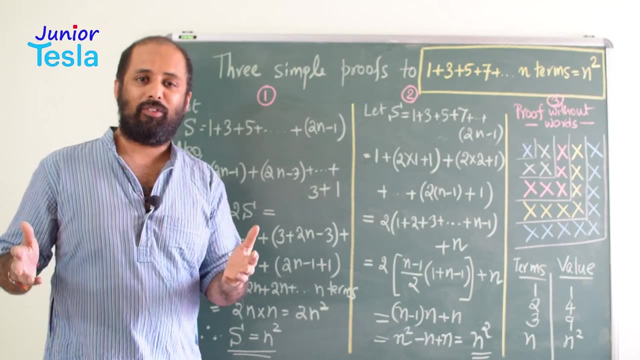 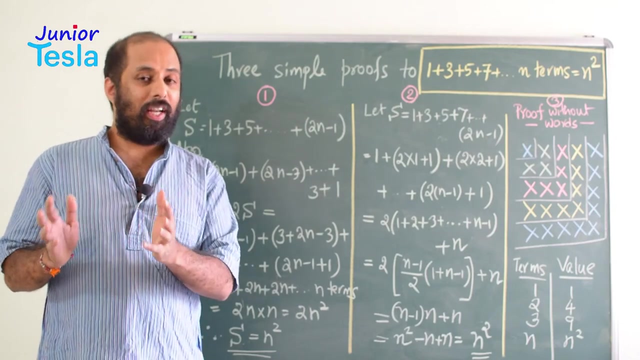 it is equal to 2s, and on the right hand side you have 2n square. Therefore, yes, equal to n square. Now, what is yes? Sum of first, n odd natural numbers, and that is equal to n square. This is one way, one method of proving that sum of n odd natural numbers is equal. 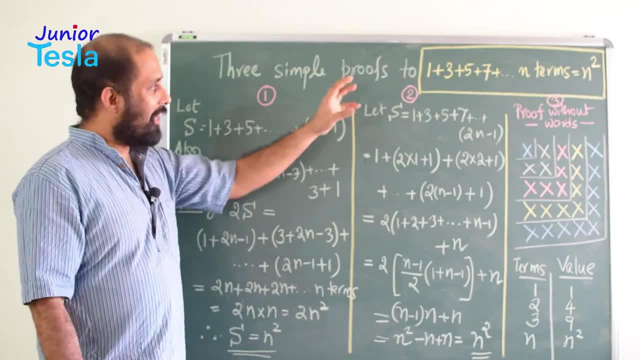 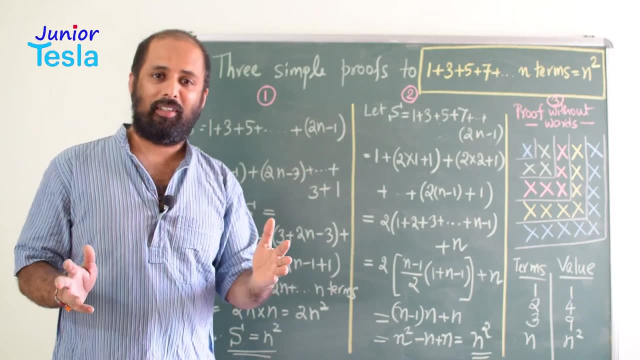 to n square. Now let us see how we can do this, how we can prove the same result in a different way. So what we do? here again, we will take series s equal to 1 plus 3, etc. up to 2n minus 1.. Now 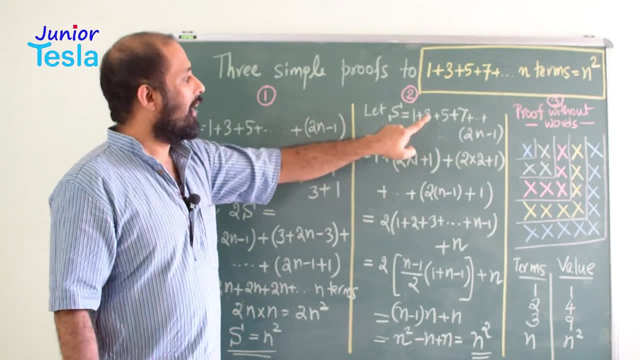 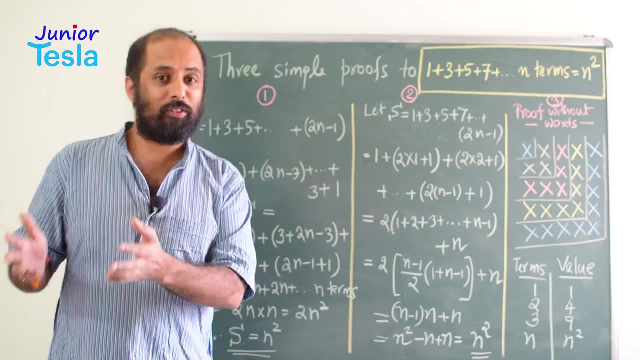 you can see some speciality here in these odd natural numbers. 3 is actually equal to 2n plus 2 into 1 plus 1.. Now 5 is 2 into 2 plus 1.. 7 is 2 into 3 plus 1.. So in general, 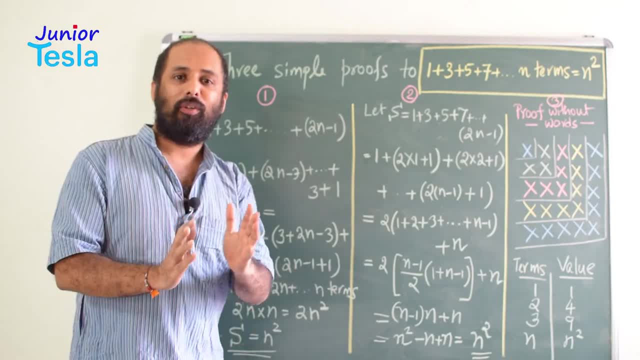 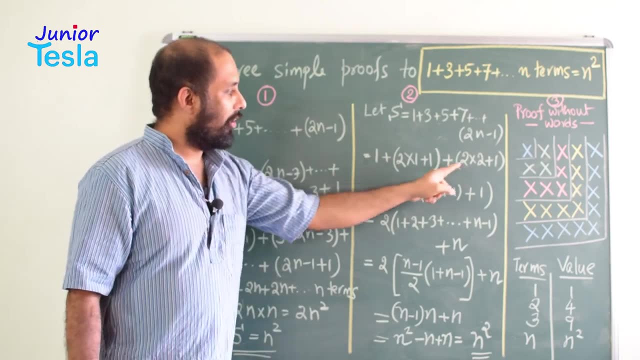 if you have taken the last term, 2n minus 1, it is 2 into n minus 1 plus 1.. Now let us use this property Here. 2 is common. In all these terms, 2 is common, So I have taken it out. and what is? 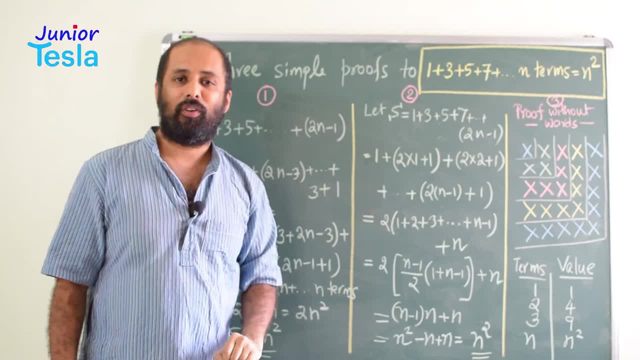 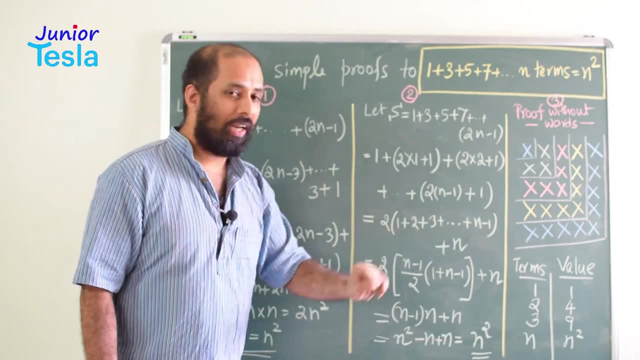 remaining is 1, 2, 3, 4, etc. up to n minus 1, and that is what I have written here: 2 into 1 plus 2 plus 3, etc. up to n minus 1, and then these 1s must be added 1 plus 1 plus. 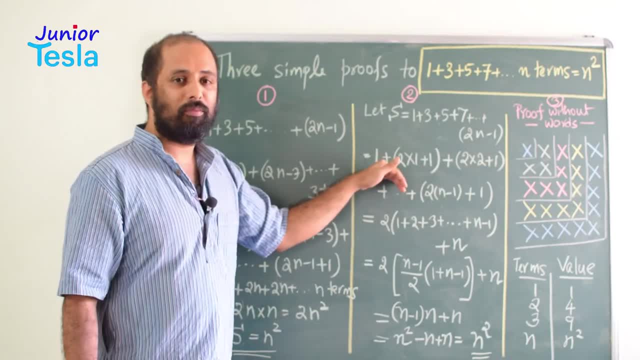 1.. So every term we have 1.. There are total n terms, So n into 1 is equal to n. So this entire expression: igtcl, lol, Show value, wooz wing. I am considering that point r to 1.. We did it superlative every time, So we have one power d Yes. what we 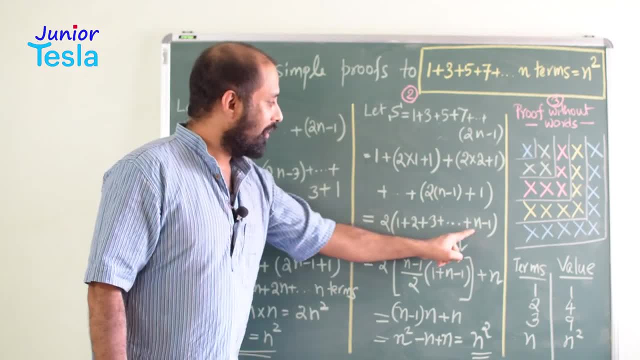 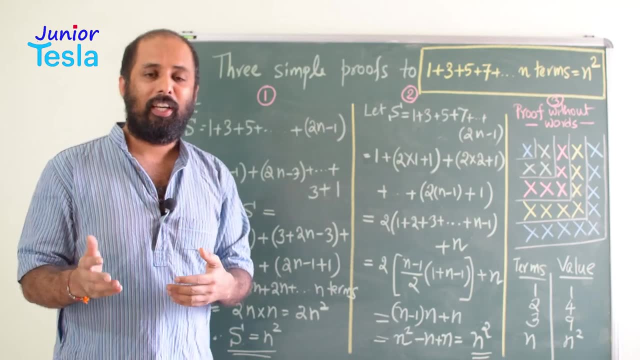 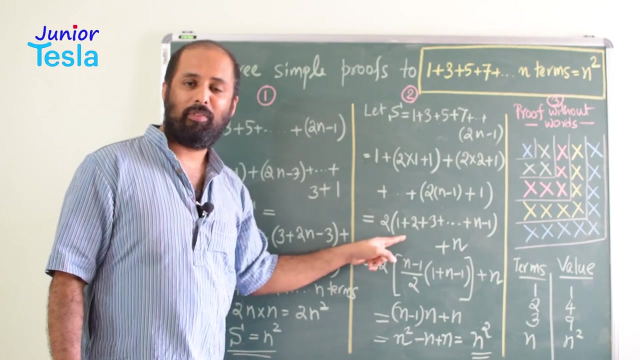 expression. Now here this is the sum of all the natural numbers from 1 to n minus 1.. We have a formula that is first number plus last number into total number of terms divided by 2.. Now here the first number is 1, the last number is n minus 1, the total number of terms is n minus 1.. Therefore, 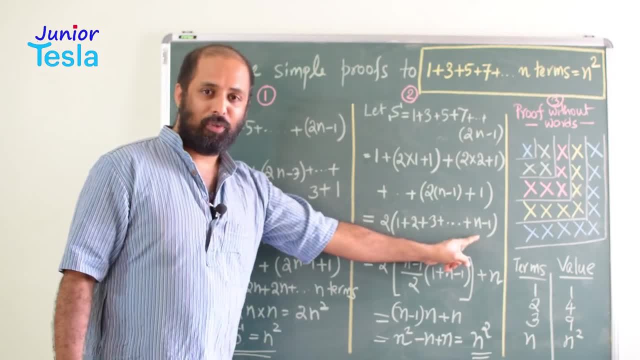 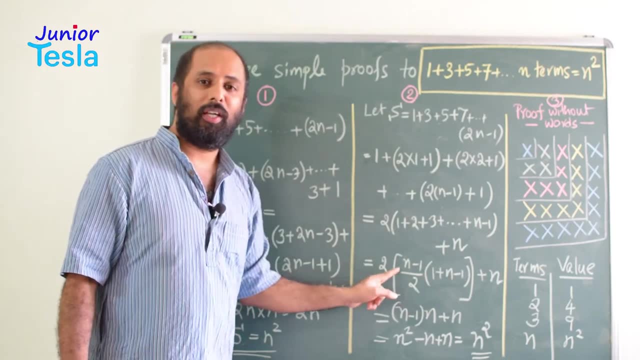 the formula says 1 plus n minus 1 into n minus 1 divided by 2.. So that is what we have written here: 1 plus n minus 1 into n minus 1 divided by 2.. That is the total sum of this particular series. 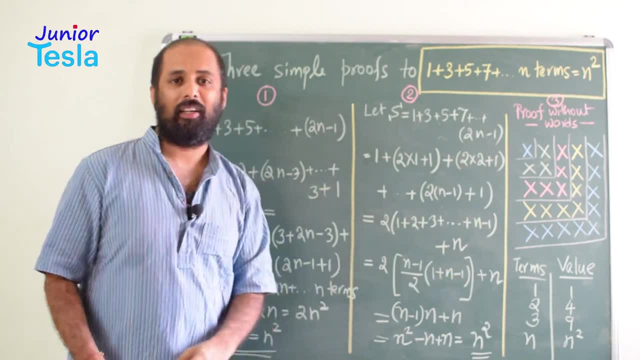 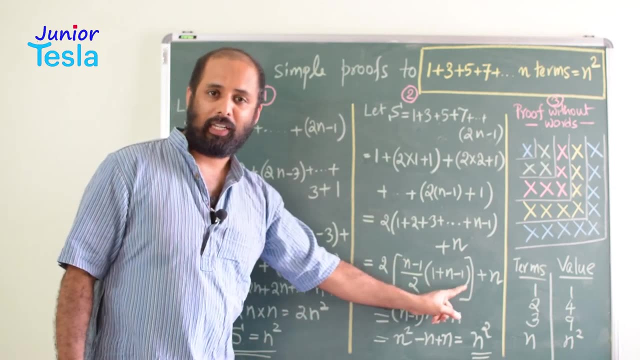 Now that into 2 and then this plus n should be written Now, if you simplify this, here 2 and 2 will get cancelled, and n minus 1 into here. plus 1 minus 1 will get cancelled, So only n is remaining. 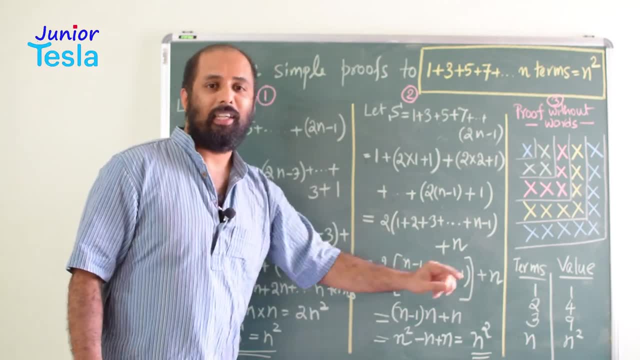 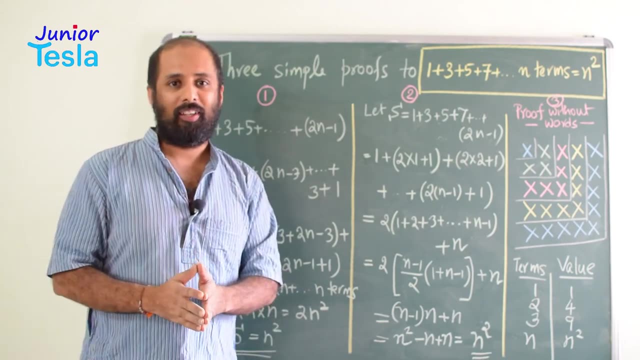 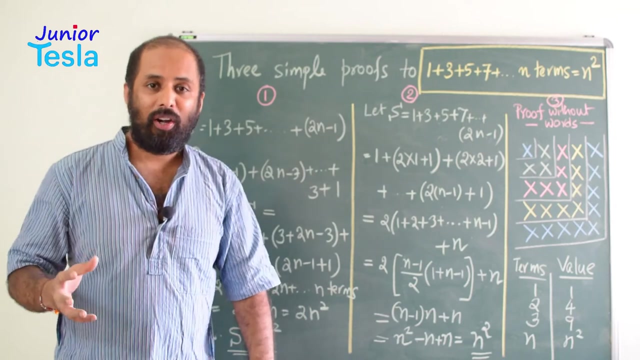 So n minus 1 into n, then plus n, which is nothing but n square minus n plus n, or it is equal to n square. So finally we are left with only n square and that is equal to S, and S is nothing but the sum of odd. 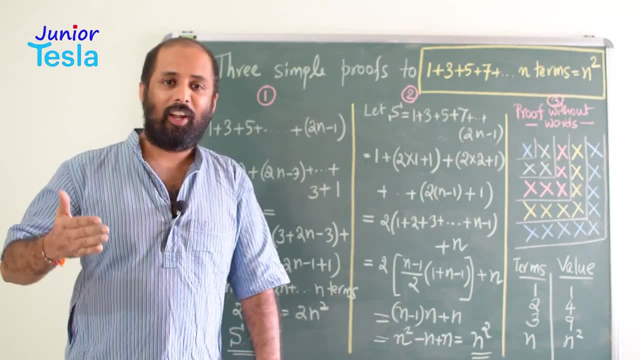 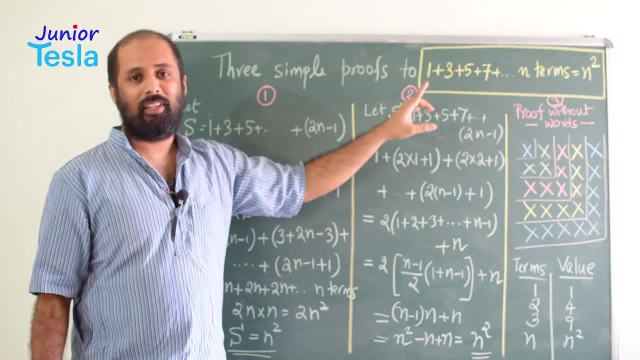 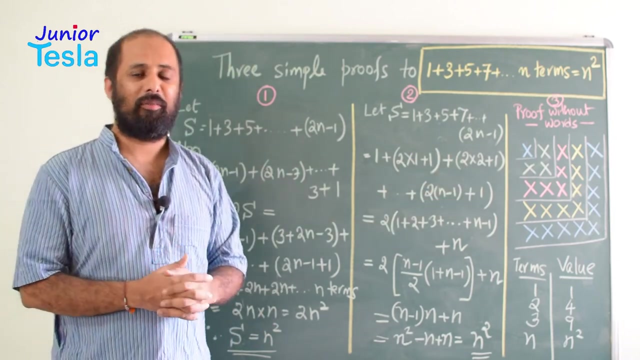 natural numbers. So if you have taken first n odd natural numbers, the sum is n square. So we have proved this theorem, this particular result, in a different way. second method. Now let me take you to the third method, which is very interesting method of proving. It is also called as proof. without words, or picture without words. So let me take you to the third method, which is very interesting method of proving. It is also called as proof without words or picture without words. So let me take you to the third method, which is very interesting method of proving. It is also called as proof without words or picture. 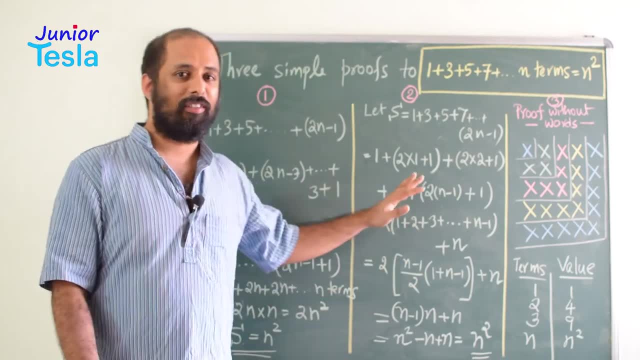 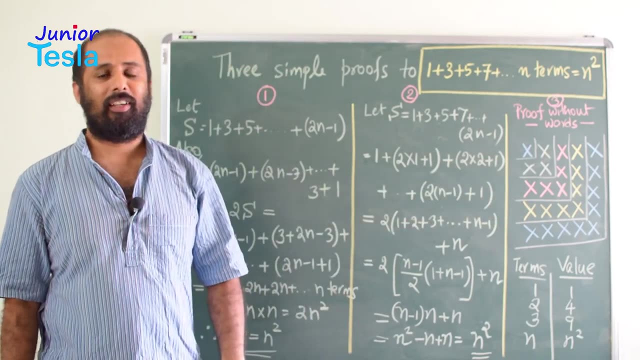 So here what we are doing is, We are not writing any equation, No algebra, no expression, no x, y, z, nothing. So here what we are doing is, we are writing some simple figures. So here we can write a bubble or a crossmark or a plus mark. 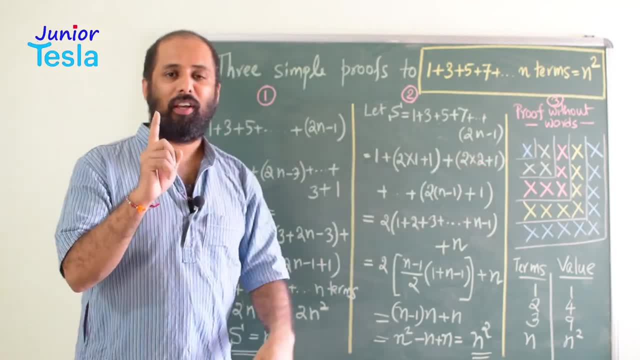 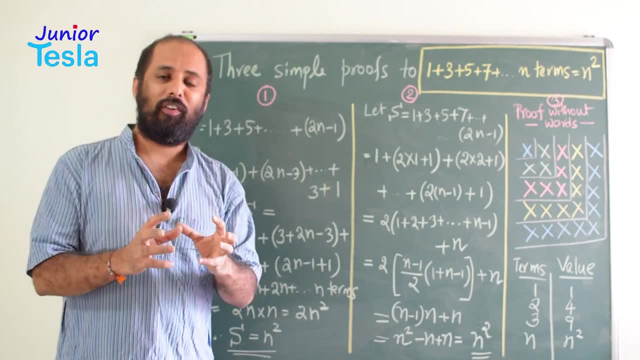 Anything. So this represents one term. so if you have take only one term, that is 1, then the sum is 1. but now, if you take 2ses, 2 terms, 1 and 3, Now you have taken 2 terms, 1and 3.. So this is 1.. This is 3.. Now, this is in the fourth, the second term, which is 2.. 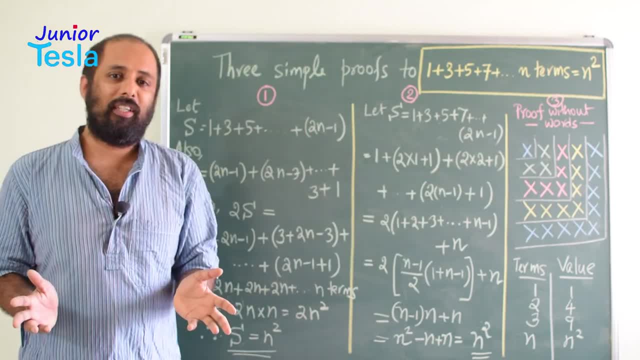 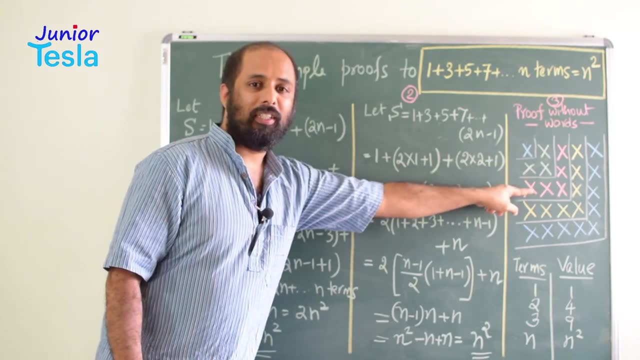 Now this is in the form of 2 by 2 square, that is, 2 by 2 is nothing but 4, 2 into 2, 4.. Now if you have taken 3 terms, so first term, second term, third term, 1 plus 3 plus 5, that 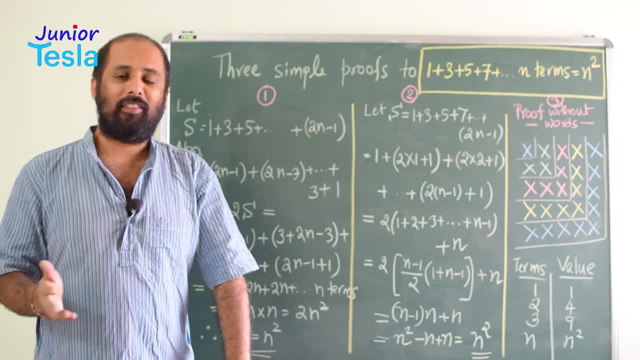 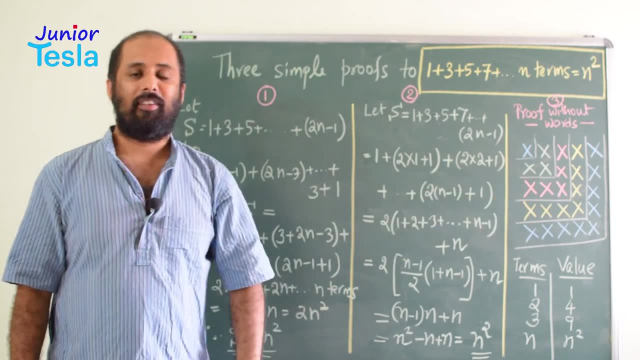 is in the form of 3 into 3,, 3 by 3 square, which is equal to 9.. Similarly, if you have taken the 4 terms, 1 plus 3 plus 5 plus 7, that is equal to it. 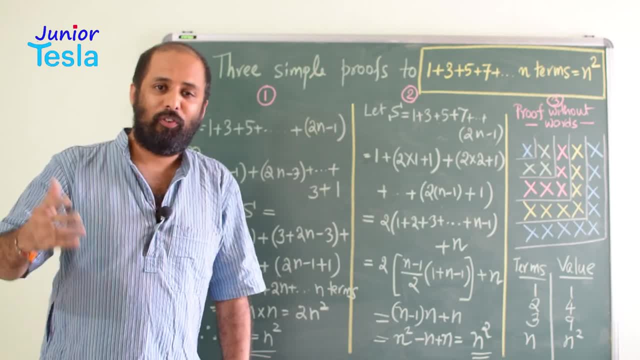 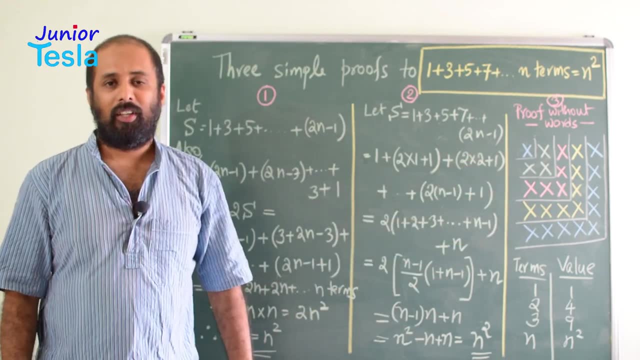 is in the form of 4 by 4 square, that is, 4 into 4, which is equal to 16.. And if you have taken 5 terms, this actually this figure, it shows 5 terms: 1 plus 3 plus. 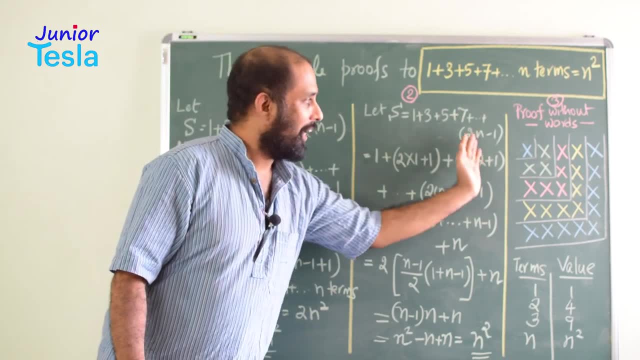 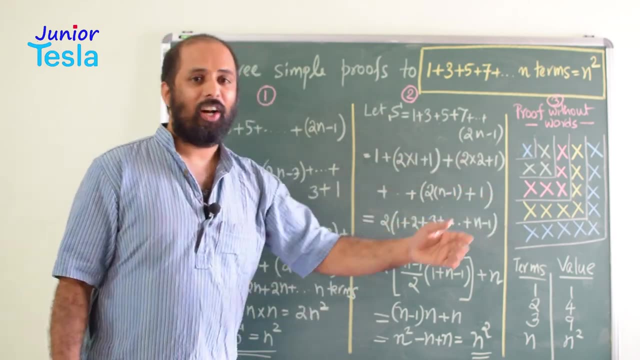 5 plus 7 plus 9, which is equal to 5 and 5.. So it is a square. 5 into 5 is equal to 25.. So in general, if you have taken n odd natural numbers, the sum is n square, and that is how. 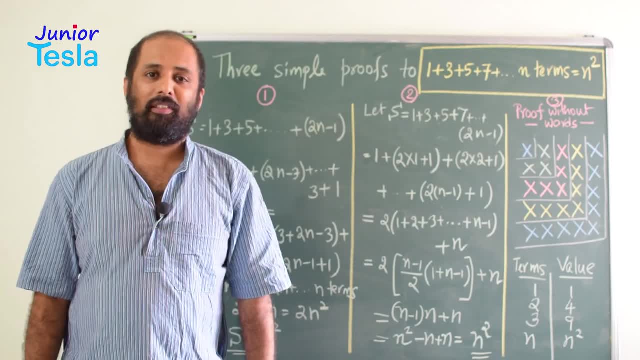 we establish this result, So 1 plus 3 plus 5 plus 7, etcetera, totally n odd natural numbers. the sum is n square, Thank you.